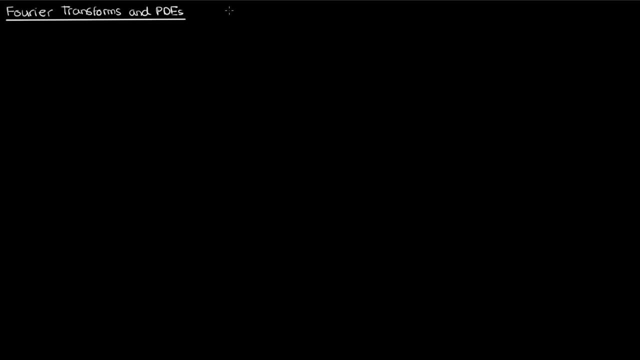 useful for PDEs with semi-infinite spatial domains, that is, where x varies from 0 to infinity. Fourier transforms, on the other hand, are particularly useful for PDEs on infinite spatial domains, where x can go from negative infinity to infinity. The first part of my video will be an introduction to the idea of Fourier transforms. 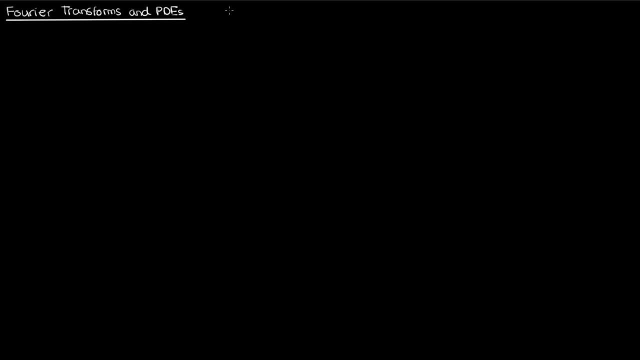 It'll be very similar to the introductory part in my Laplace transforms video. For those of you being introduced to the integral transform concept for the first time, I encourage you to watch this introduction, And for those of you who've already seen my Laplace transform video, I'll put a timestamp in the description to skip this first one. 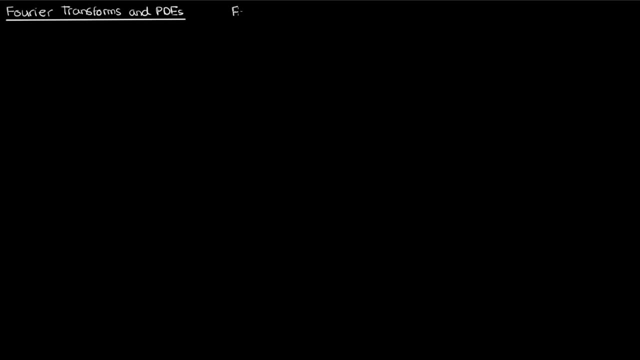 Now, what is the Fourier transform? Well, it's a special type of integral transform. Its job is to transform a function using an integration operation. Essentially, it changes a function, f of x, to another function- f hat of omega- using this integration formula, where f hat of omega, the Fourier transform of f of x, is the 1 over the square root of 2 pi times. 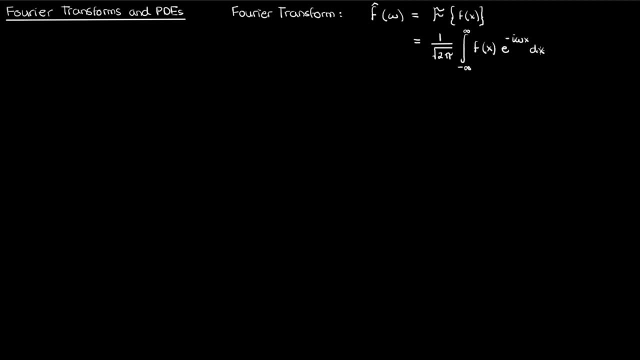 the integral from negative infinity to infinity of f, of x times the exponential of negative i. omega x with respect to x. The i, of course, is the imaginary number. here The Fourier transform is also invertible, which means I can take my f hat of omega and get f of. 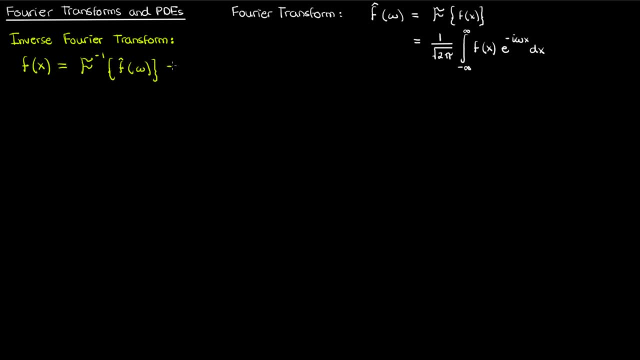 x from it using something called the inverse Fourier transform, which I can find using the 1 over the square root of 2 pi times the integral from negative infinity to infinity of f. hat of omega times the exponential of i, omega x with respect to omega. 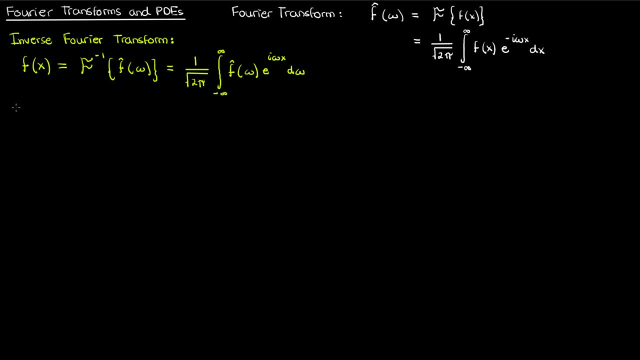 So these equations for the Fourier transform and its inverse are all fine, but let me explain why the Fourier transform is useful when solving both odEs and pDEs. If I have an ordinary differential equation like the second derivative of f with respect to x is some function g of x, f and df by dx, then because the Fourier 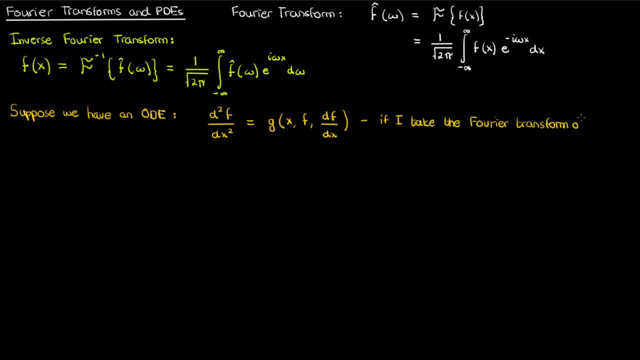 transform is an integral transform. you can intuitively imagine that if I apply the transform to this differential equation, I will in fact integrate out one of the variables. In this case, if I integrate out the x with respect to one of the variables, I can integrate one of the variables. 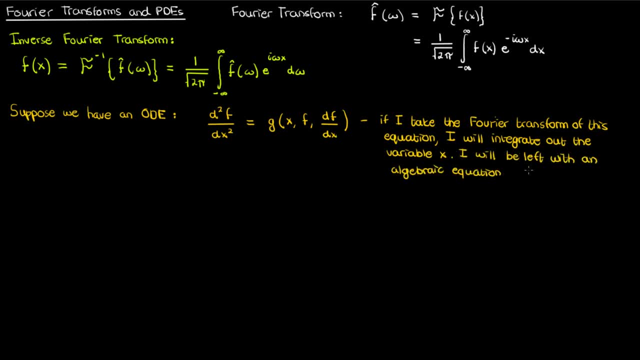 completely. I won't be left with any derivatives and in the end I'll just be solving an algebraic equation for the Fourier transform of f- hat of omega, which is the Fourier transform of f of x. Now, once I've solved this algebraic equation for f- hat of omega, I can take the inverse transform. 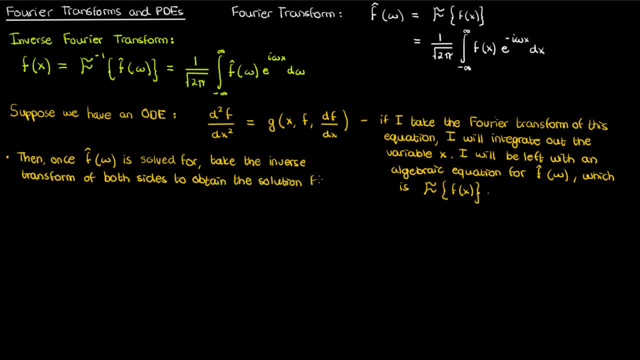 of both sides to get the solution for our function f of x. The inverse transform essentially converts a Fourier transformed function f hat of omega to the original function f of x. This inverse transform stage is often the hardest part because there's a lot of work that goes into manipulating. 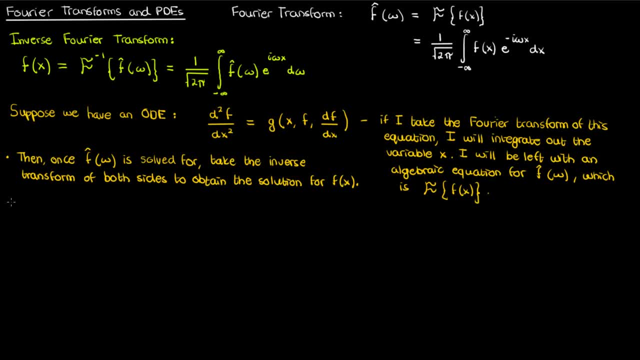 f hat of omega, so that we can eventually find the inverse transform. In addition, there's a lot of complicated functions out there whose inverse transforms are nearly impossible to find. Now, what about for partial differential equations? Well, suppose I have a partial differential equation, like the one-dimensional heat equation, which involves a function u. 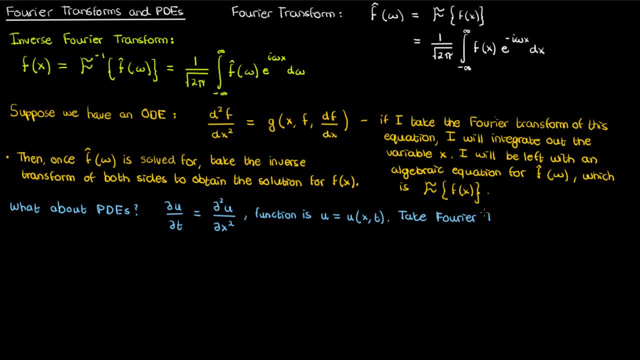 of x. Now, what about for partial differential equations? Well, suppose I have a partial of x comma t. Now what I can do is take the Fourier transform of this PDE with respect to the position variable x and, as I mentioned before, when I take the Fourier transform with respect to: 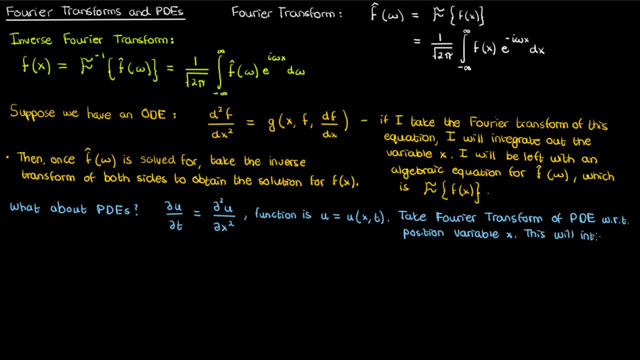 an independent variable which is an integral transform. it's as if I'm integrating out that independent variable. So when we integrate out the x in this PDE, we'll be left with a differential equation in t which is simply an ODE Again. once I solve this ODE, I'll end up with a solution. 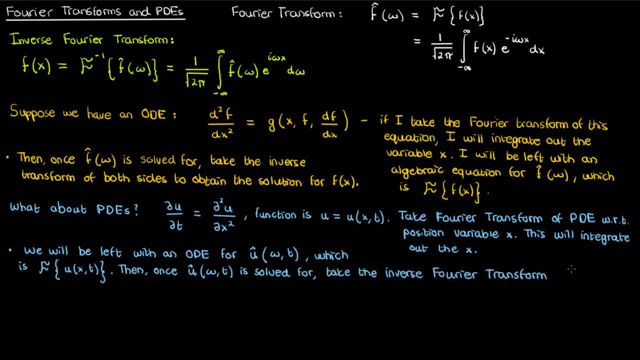 for u hat of omega comma t, which I can use to get u of x comma t, by taking an inverse transform. By a similar logic, if my PDE involves partial derivatives and n independent variables, then taking the Fourier transform of that PDE with respect to one of those independent variables. 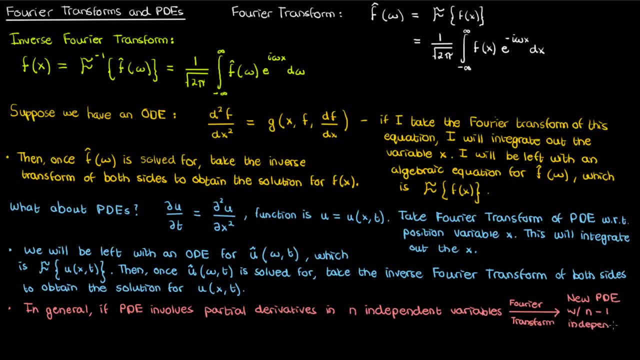 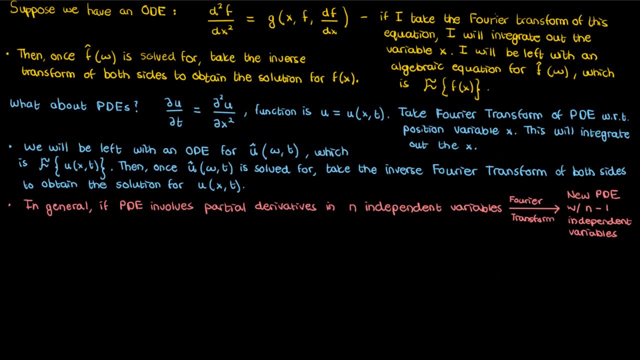 will result in a new PDE with n minus one independent variables, because again the Fourier integral transform integrates out one of those variables. As a result, the Fourier transform may be a new PDE with n minus one independent variables, because again the Fourier integral makes our differential equation simpler Again. the hardest part is usually at the last step, when you 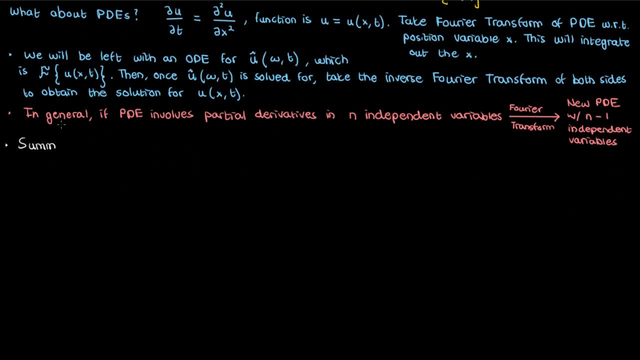 need to find the inverse Fourier. Now, for ease of reference, I'm going to summarize the Fourier transform process right here. So we start off with a differential equation involving the function u of x. u could still depend on other independent variables like y, z and t, but I've only written. 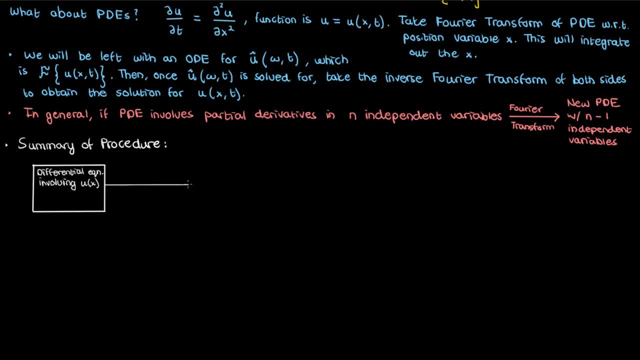 down x, because that's what we're Fourier transforming. Then what we do is we take the Fourier transform of this differential equation to end up with a simple differential equation. We start off with a simpler equation involving u hat of omega, the Fourier transform of u of x. 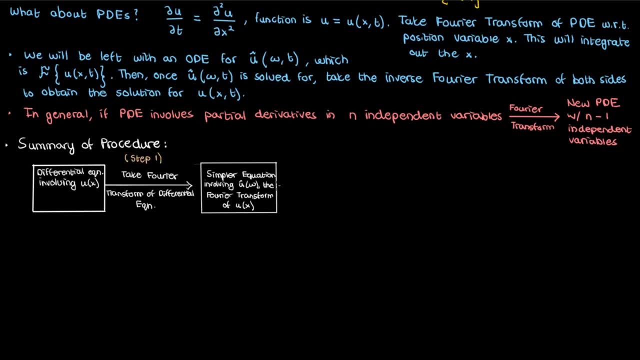 This is step one. Now, this equation could be an algebraic equation, it could be an ODE, it could be a less complex PDE, as we just discussed, but the idea behind this equation is that it's easier to solve than the original differential equation. In step two we're going. 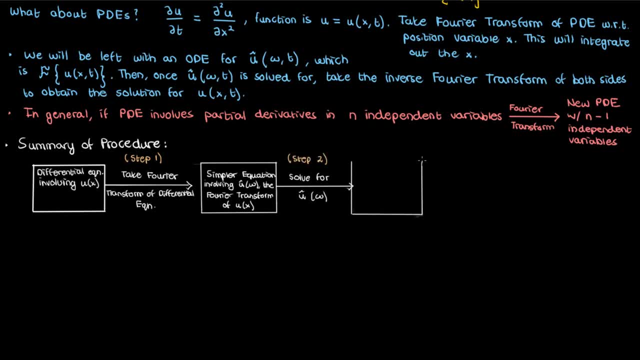 to solve the simpler equation, to end up with an expression for u hat of omega. and finally, in step three, we'll take the inverse transform of u hat. and what happens when we take the inverse transform of u hat? Well, we'll end up with an explicit equation for u of x. Now, before we get, 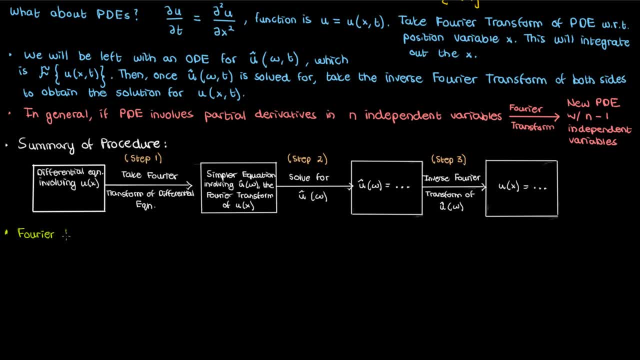 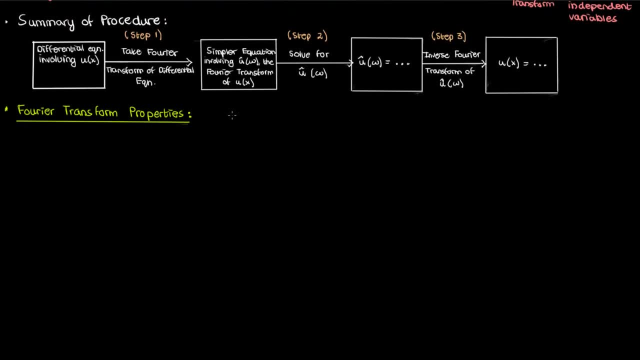 to solving PDEs using Fourier transforms. I want to quickly go over some properties of the Fourier transform, particularly when it comes to the derivatives of a function. Now say I have a function u of x, comma, t, and I'm taking its Fourier transform with respect to x and say that the Fourier 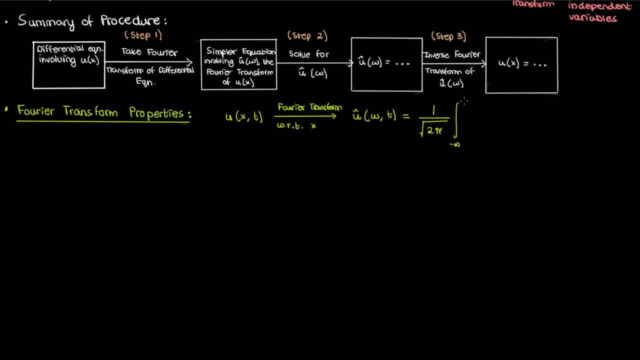 transform of u is u hat, which is given by this integral. per the definition of the Fourier transform, Suppose that I want to find the Fourier transform of the nth partial of u with respect to x. To find this Fourier transform, I'll have to use the fact that the nth derivative of u with respect to x. 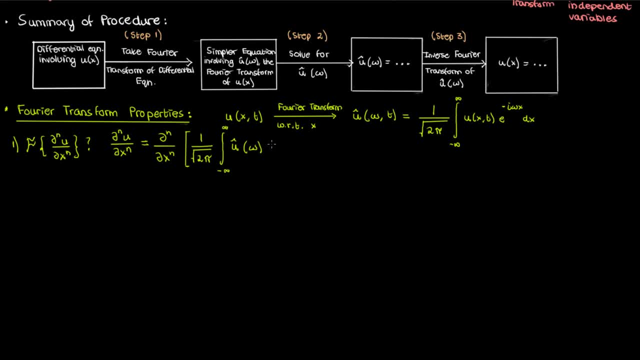 is the nth derivative of the inverse Fourier transform of u hat. That makes sense because u is pretty much equal to the inverse Fourier transform of the Fourier transform of u. so the inverse Fourier transform of u hat. Now, since the integral on the right is integrating out the omega and not the x, it. 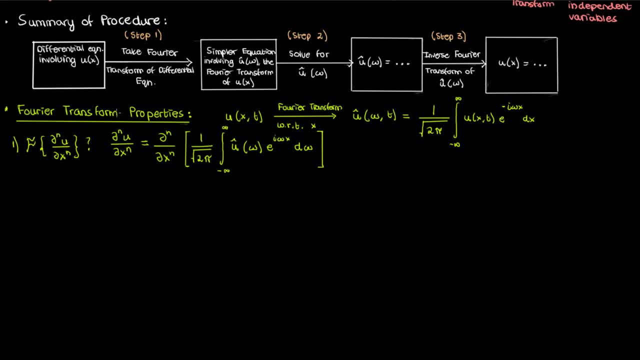 with d omega at the end. after all, and since u hat should be continuous and differentiable, we are allowed to differentiate under the integral sign. But the nth derivative in x inside this integral is just the nth derivative of the exponential. since the u hat doesn't contain x, it's only got. 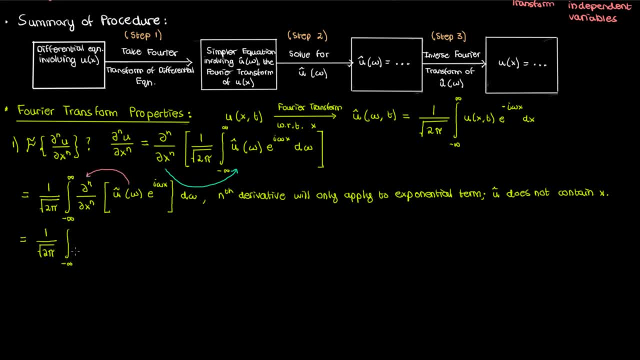 the omega. so u hat is basically a constant as far as this derivative is concerned. And when you calculate the nth derivative of the exponential with respect to x, you'll still get the same exponential, but the i omega will come out front with each derivative. so if you differentiate n, 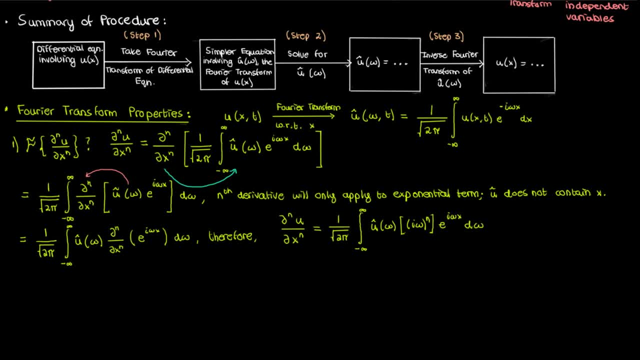 times, the i omega will come out n times. so this is what we'll end up with. And finally, based on the definition of the inverse Fourier transform. if you have to take the inverse Fourier transform of this function to get the nth partial of u with respect to x, that would mean the Fourier. 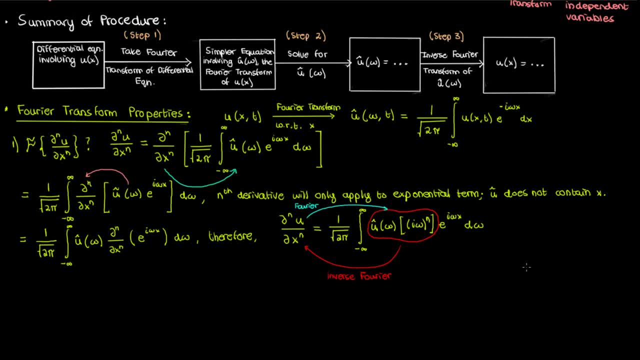 transform of the nth partial of u is then this function that I've circled, Therefore the Fourier transform of the nth partial of u with respect to x, where x is the variable that's being integrated out in the Fourier transform. the Fourier transform is given by i omega to the n times the Fourier transform of u alone, which is just our u hat. So this is: 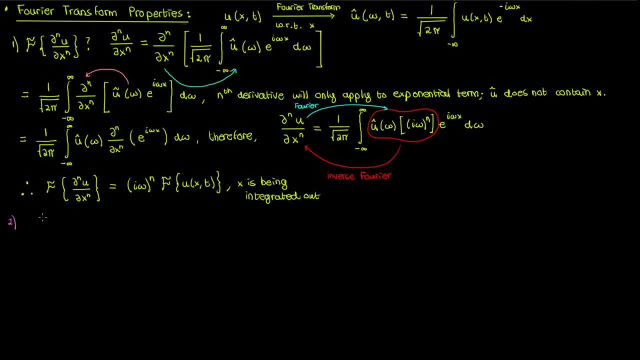 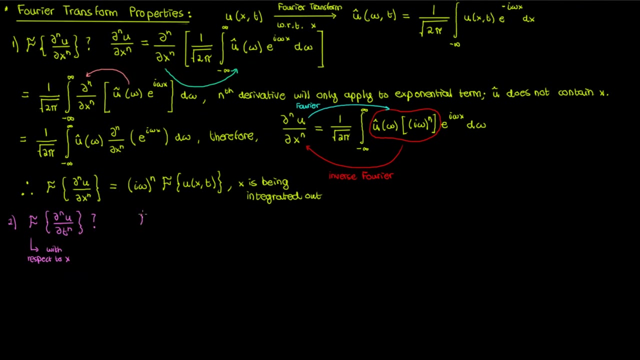 the first property of the Fourier transform. Let's discuss the second property, which is the Fourier transform of a derivative with respect to the variable that's not involved in the transform. So in this case we're Fourier transforming with respect to x, but our derivative is with respect to t. This should be a relatively quick derivation. 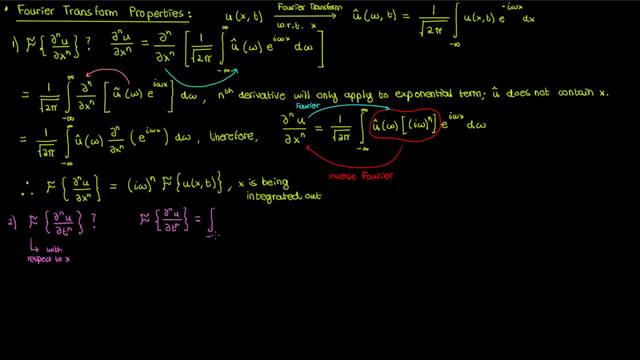 By the definition of the Fourier transform. the transform of the nth time derivative of u is given by the following: And since I'm not integrating with respect to t, I can take this time derivative outside the integral, since the time derivative is irrelevant to our integration. Now the integral. 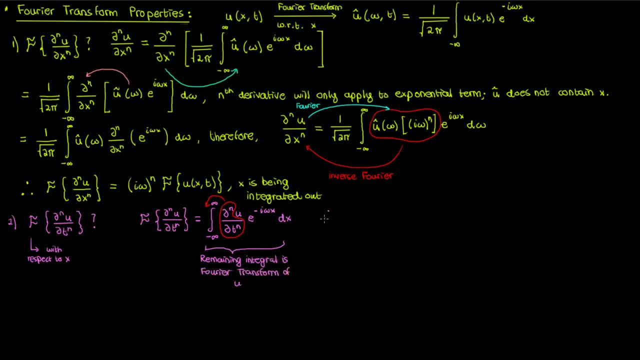 that's left inside is just the Fourier transform of u. So the Fourier transform of the time derivative of u is the time derivative of the Fourier transform. Again, time is the variable that's not being integrated out in the Fourier transform. The third and final property of Fourier transforms that I'll discuss here is the convolution. 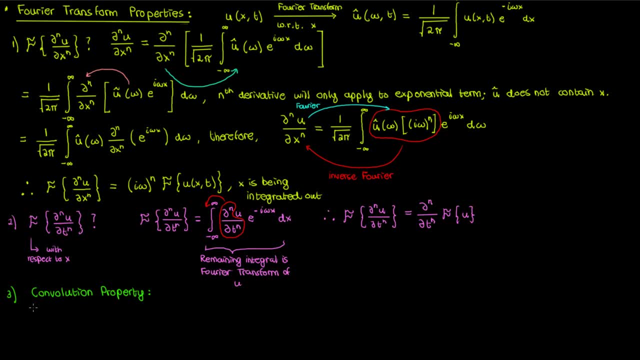 property which is based on the convolution theorem. It states that the Fourier transform of the convolution of two functions is the product of their individual Fourier transforms. I've stated this property without proof here, but if you want the proof, you can head over to my introductory video on convolution Links in the description. Now I'm going to spend. 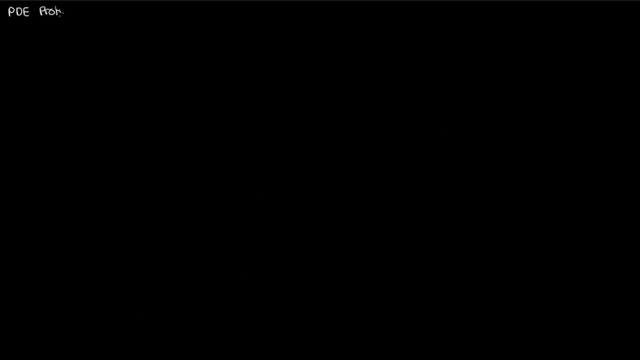 the rest of the video using the Fourier transform to solve a simple PDE problem. Suppose that you have a rod of infinite length with an initial temperature distribution of phi of x. Suppose also that heat is transmitted along this rod only by conduction. so the PDE governing 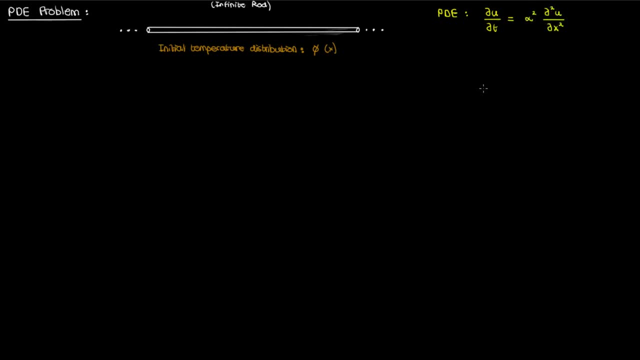 the transfer of heat along this rod is given by the typical heat equation, where alpha squared is the thermal diffusivity of the rod and u is the unknown temperature distribution at time t. Since the rod is infinite, there aren't any boundary conditions, so we only 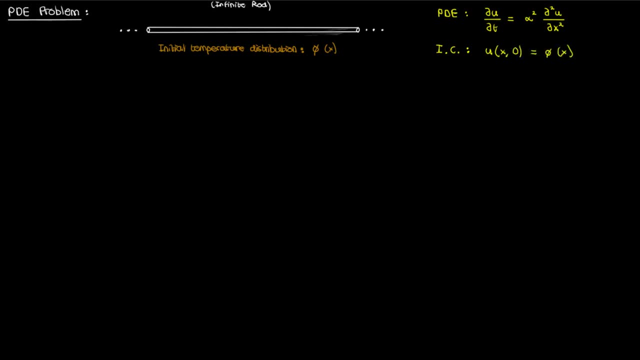 have the initial condition that the temperature distribution at time zero is phi of x, Since the rod is infinite. our position: variable x can vary from negative infinity to infinity and for this reason it makes sense to use the Fourier transform, because the Fourier equation integrates also from negative infinity to infinity. so we'll Fourier transform both. 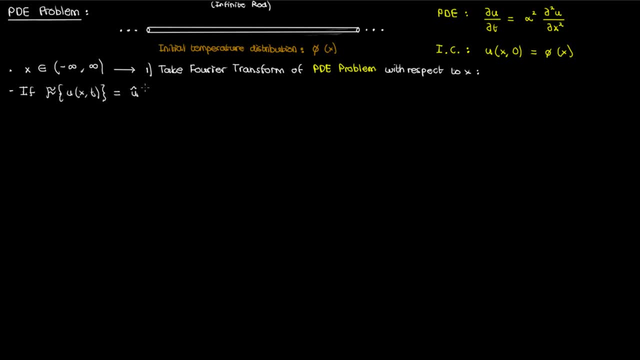 the PDE and the initial condition, Assuming the Fourier transform of u is u hat of omega comma t. the Fourier transform of the PDE is given by the partial of u hat with respect to t, equals negativecomb of x upon t squared over t squared and tau squared over phi of. 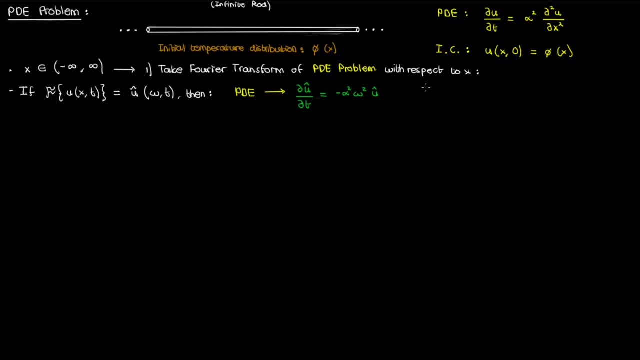 t squared over z squared over x cubed over t squared off, and you get the same operation: negative alpha squared omega squared u hat, according to the first and second properties I discussed earlier. Meanwhile, the Fourier transform of the initial condition gives me some function that I'll call psi of omega, which I'll suppose is the Fourier transform of phi of x. 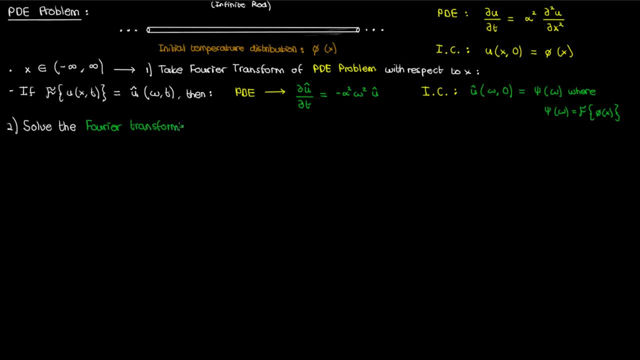 The next step is to solve the Fourier transformed problem. This actually isn't too difficult. The first order differential equation in time can be solved by separation of variables. so the dt goes on the right and the u hat goes on the left. Integrating both sides gives us the following: 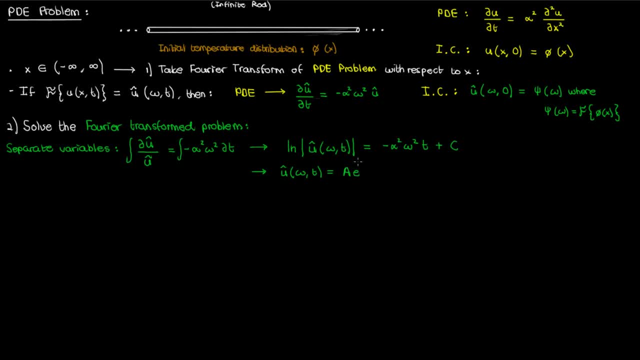 and then when I take the exponential of both sides, here's what I'll end up with, where a is just the exponential of c, And to find a I can apply the initial condition. so at t0 u hat is psi of omega, which then makes a equal to psi of omega, which means that the solution to my Fourier 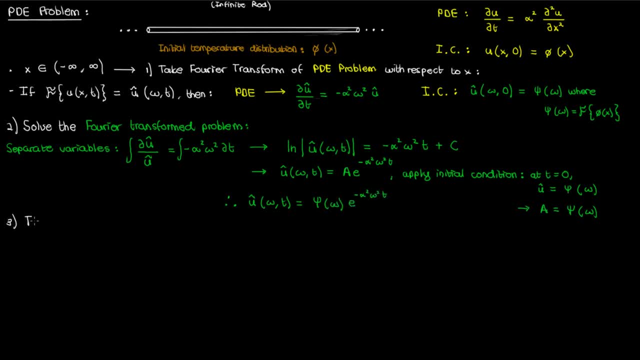 transform. PDE is the following: And this is where we'll move to the third step, which is to take the inverse Fourier transform. And if we take the inverse Fourier transform of u hat, this is what our equation will look like Now. the inverse Fourier transform on the left is just u of x comma t, but the inverse Fourier 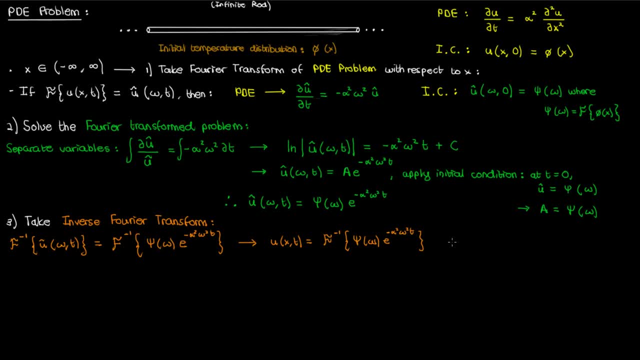 transform on the right is going to be a bit difficult to handle. There is one trick, though, we can use to make the right hand side more manageable, and that trick is the convolution theorem. From the convolution theorem, the product of the Fourier transform of two functions is: 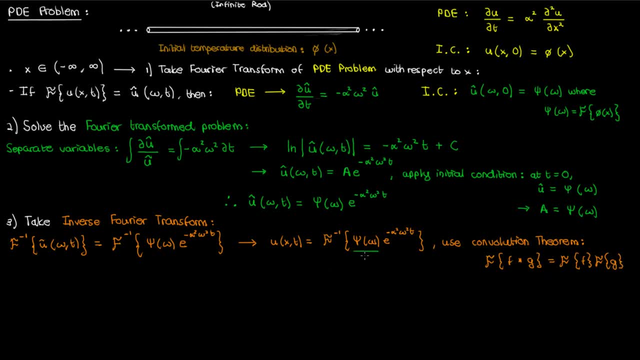 equivalent to the Fourier transform of their convolution. In this case we're multiplying the Fourier transform of phi, of x, which is psi, and this exponential, which is presumably the Fourier transform of some function that we haven't figured out yet. So by the convolution theorem we can write the product of these Fourier. 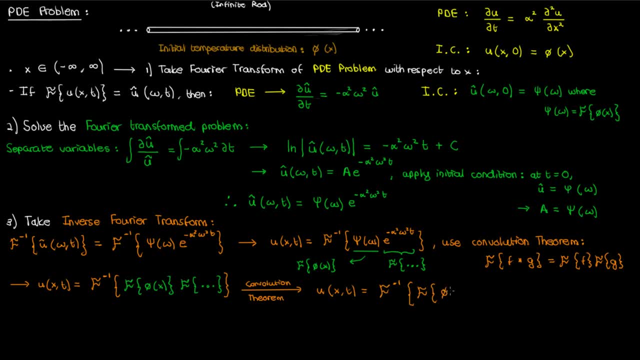 transforms as the Fourier transform of the convolution of the original two functions. and when we do that, u becomes the following: This dot dot dot, by the way, represents the inverse Fourier transform of this exponential term. and if you look it up, 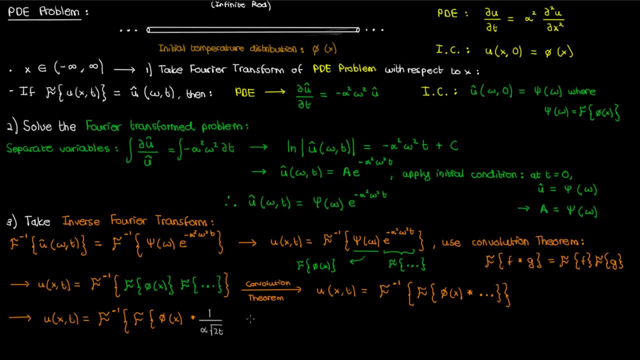 Fourier transform tables, or if you calculate it yourself, you'll find that it's equal to 1 over alpha times the square root of 2t times the exponential of negative x squared over 4 alpha squared times t. And, of course, in front of the 1 over alpha square root of 2t there's an additional. 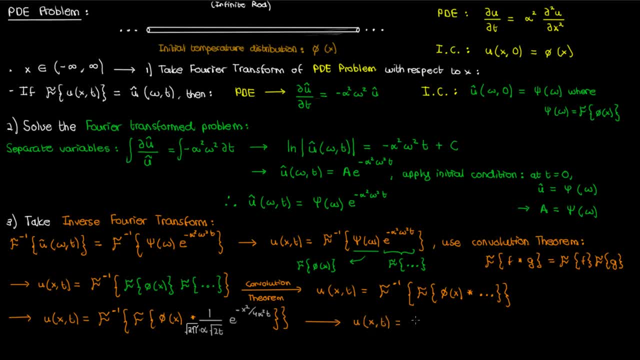 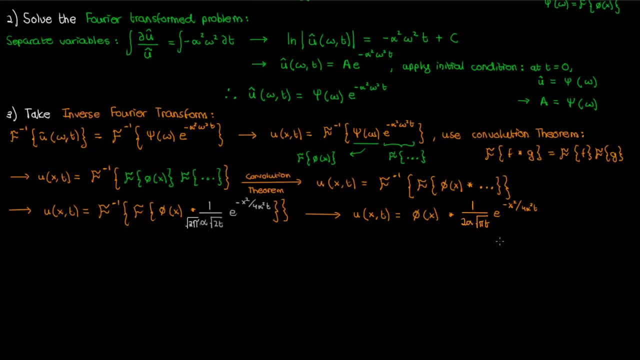 1 over square root of 2 pi, which then would make this 1 over 2 alpha square root of pi times t. out front Now the inverse Fourier transform of the Fourier transform is just the function itself. so u of x comma t is then the convolution of these two functions. Recall that the convolution. 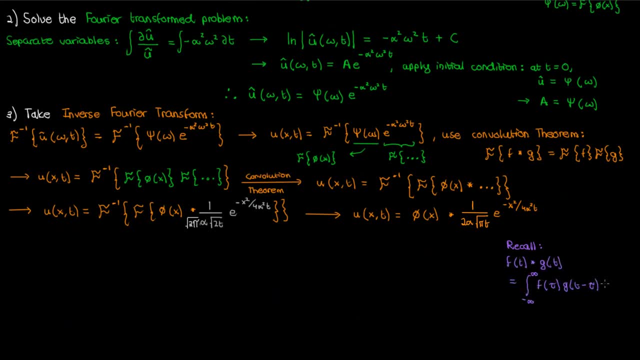 of two functions, f and g, is given by the following: where tau is some dummy variable, we're integrating over And using the definition of convolution u of x, comma, t finally becomes the following: where y is just the dummy variable, kind of like the tau in the definition of my convolution here, 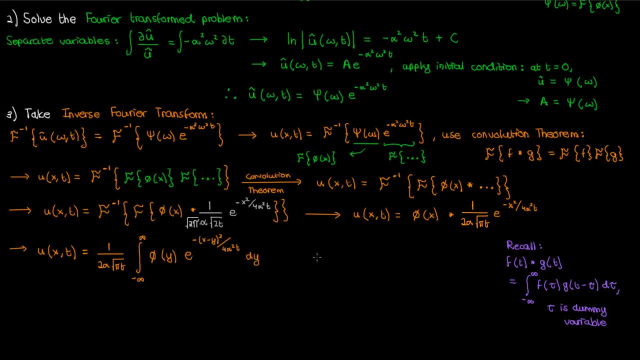 And so, in the end, this is the solution to my heat equation on an infinite rod, which I found using Fourier transforms. Before I end this video, there's a couple of important points I'd like to mention. The first is that this exponential function in the integral for u, the function 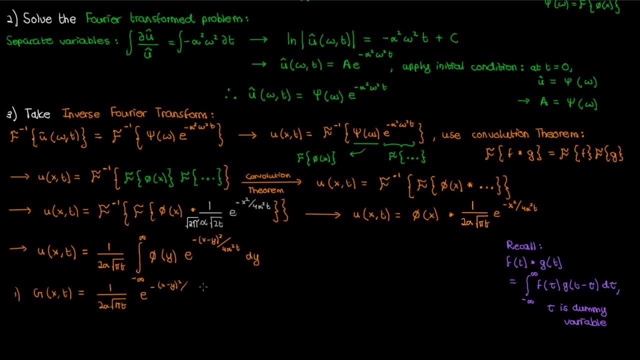 multiplying the phi along with the constant out front. this function, which I'll call g of x, comma t, is called the Green's function. The Green's function essentially describes how the PDE responds when you have a delta function input, so an impulse input. So basically, if my initial 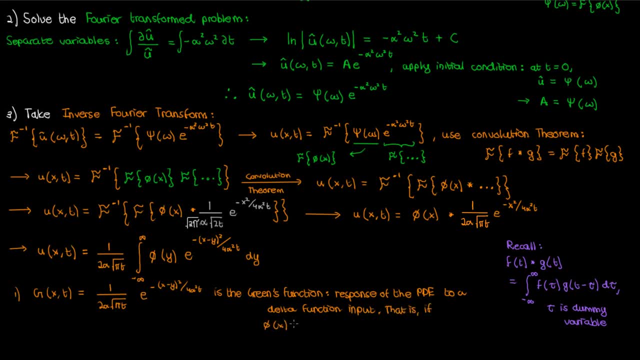 condition phi of x, which is the only input that I have for this system. really, if my initial condition was a delta function, you could show using the properties of delta functions that u of x comma t would be equal to the Green's function. If I had some more complex input, I would need to.